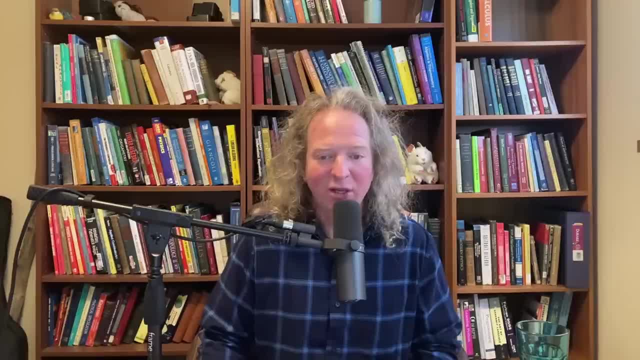 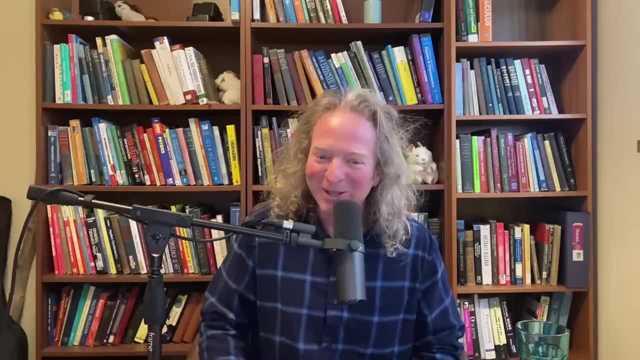 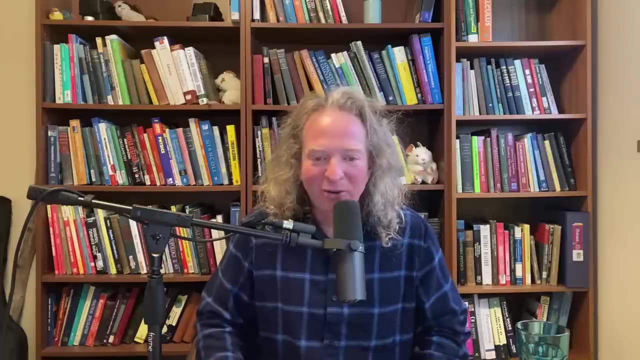 are built. I feel that all what I am reading is people showing that they know the material, that it is not that they are teaching it. I'll keep reading now, because so much rely on set theory is really difficult to keep track of what is going on and why are the steps being taken. So I am looking for a real 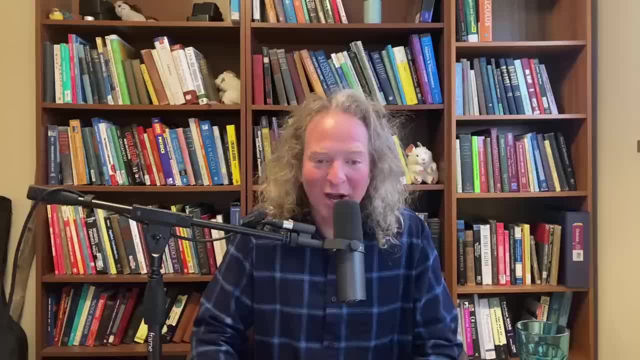 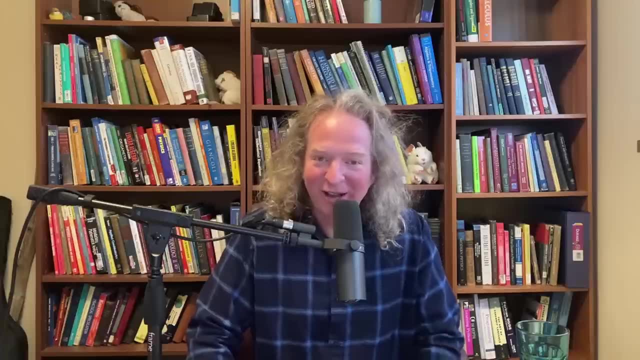 beginner's book to measure theory, and so far I have failed. That is why I am calling on your wisdom plus sorcery for help. Thanks, Leothen. So first let me say, Leothen, that I feel your pain. I know how hard it is. I took measure. 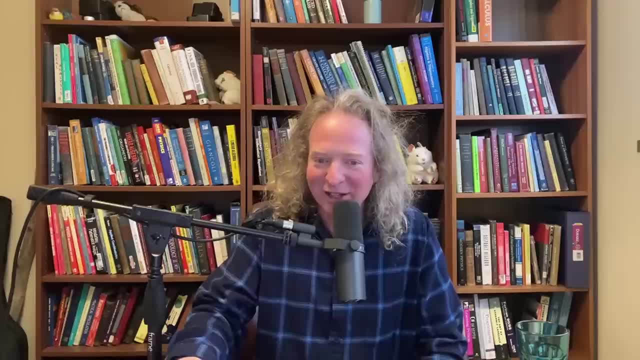 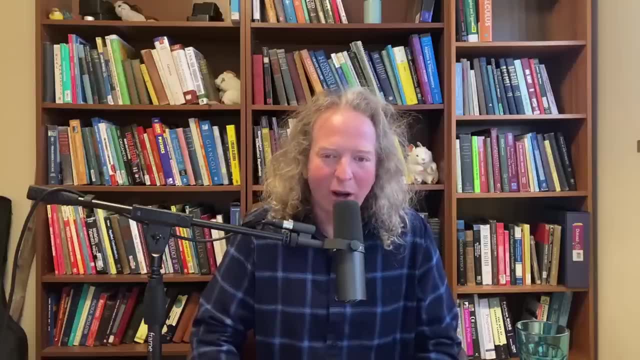 theory. It is a very challenging class, to say the least. So my advice, My advice is not to get one particular book because, honestly, I don't know of one particular book. that is like absolutely incredible when it comes to measure theory. I mean they are. 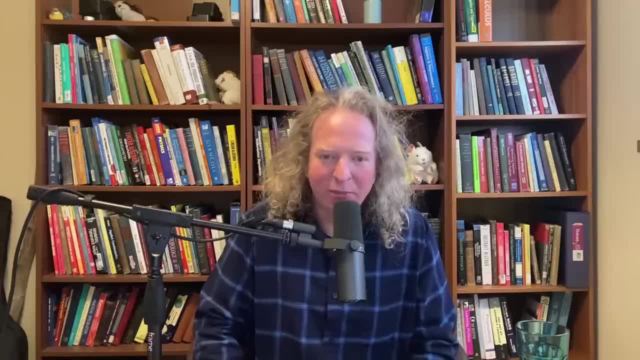 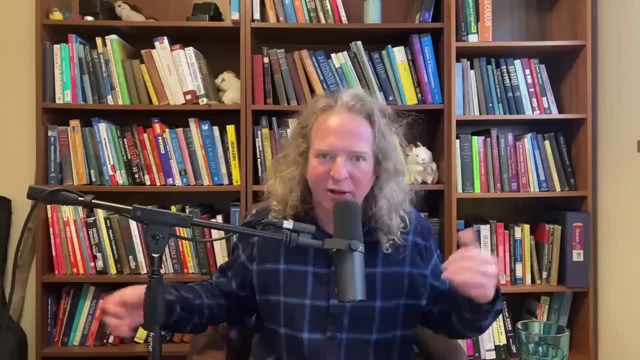 all okay. My advice would be to get as many books as possible, The books by Folland. I think the Folland book is pretty good, The book by Royden is pretty good. The book by Rudin is a classic. So Folland, Royden and Rudin, those are the classics. And there is 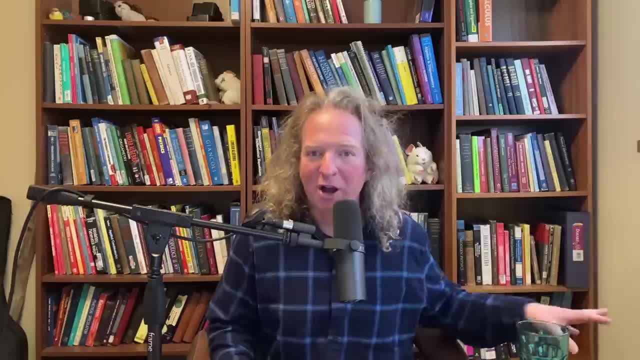 many more. Then there is another really interesting one. So this stuff hilarious. and I have other real analysis books from other authors you've probably never heard of. So my advice would be to just get as many books on the subject as you can. 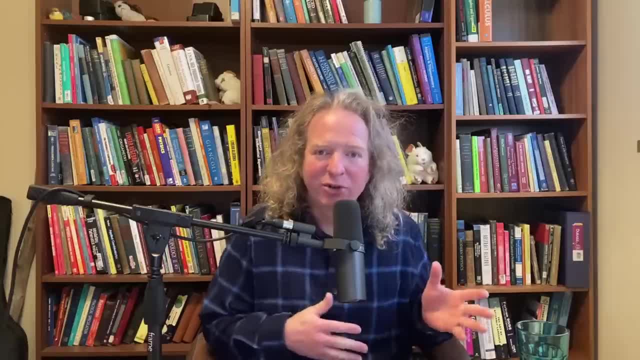 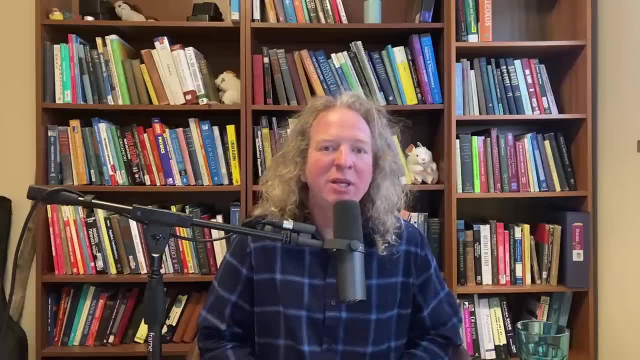 And then when you are going over this stuff in your class, like I am sure you have a lecture, So you have your lecture, You write down your notes, Make sure to go over your notes. and when I say go over your notes, I mean like go over your notes, like spend a couple hours. 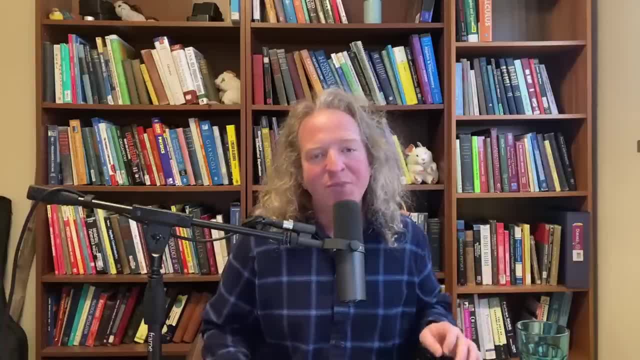 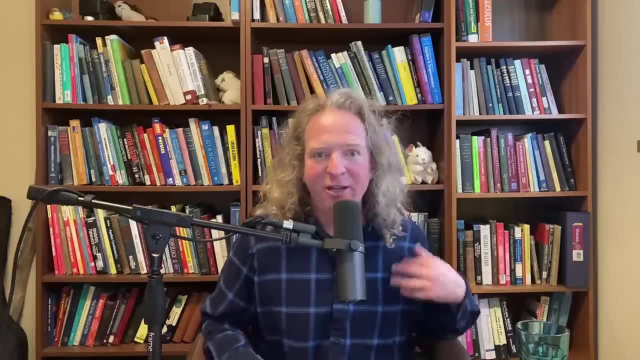 right after class, whatever it takes going over your notes. Then if there is stuff you don't understand from your notes, Kit, go see your professor if they have office hours, or go see a ta if you have a ta, if not, that's okay. 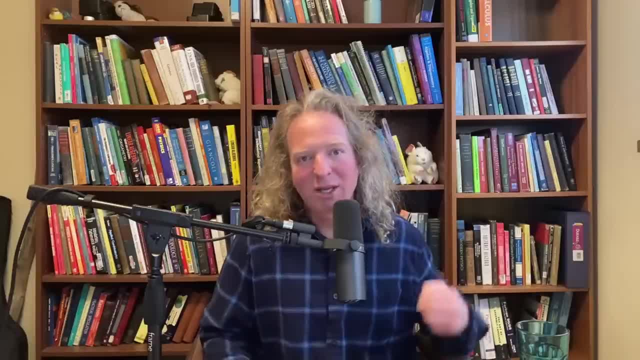 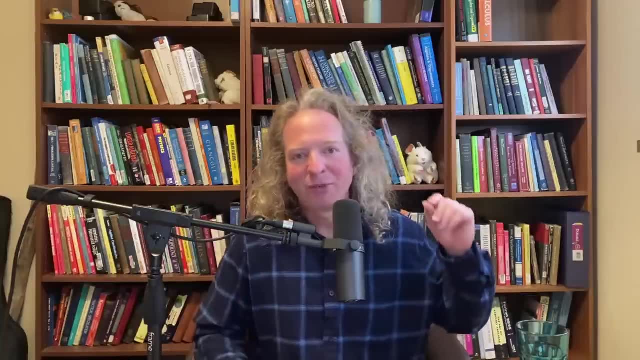 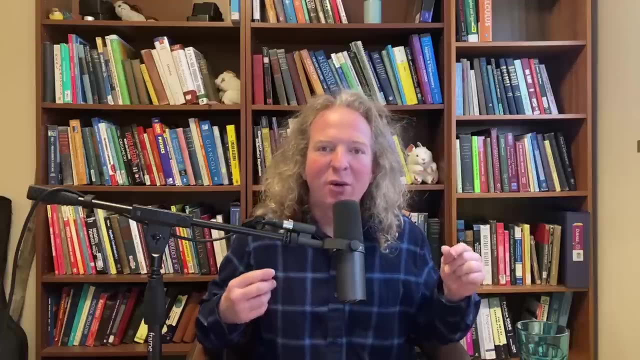 you're still doing the best you can, and that's important. i think it's that you do the best you can. so surround yourself with tons of books again. you can get them super cheap and go over your notes a lot. then, when it comes time for the test, what i used to do in real analysis is i wouldn't. 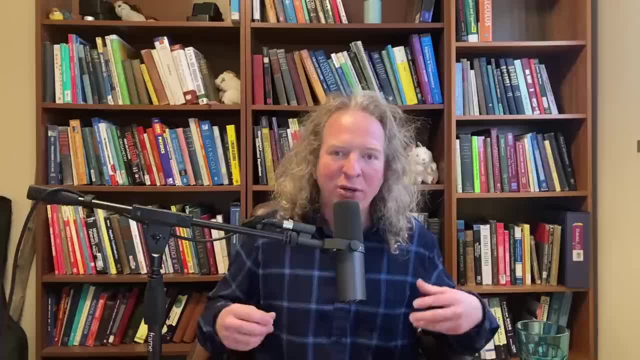 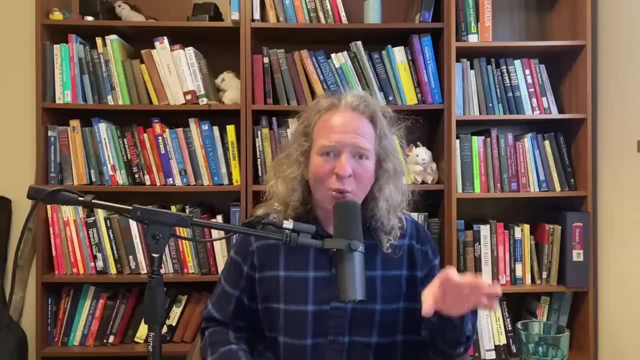 just go over my notes, because i didn't always understand everything, and i wouldn't always just go over the homework, because sometimes i didn't understand all of that either. i would also do problems from other books, so you want to do exercises and example problems from other real 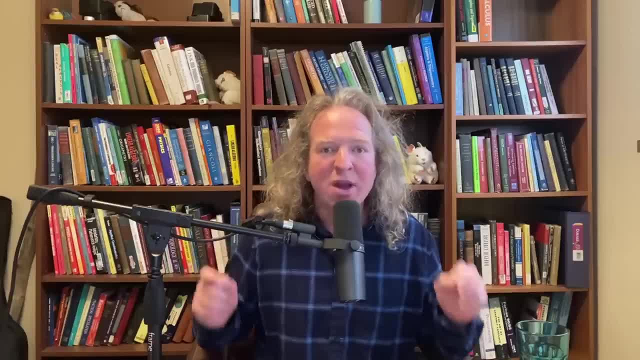 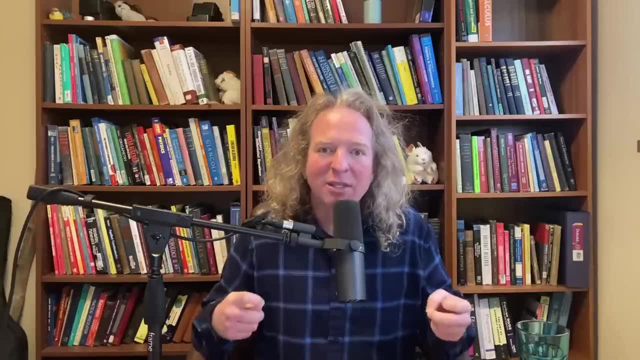 analysis books again. get as many as you can and do as many problems from different books, because that's how you learn right. that's how you learn analysis. that's how you learn math. it's by doing problems. and you're right. you made that comment and made me laugh. it said: let me see if i can find. 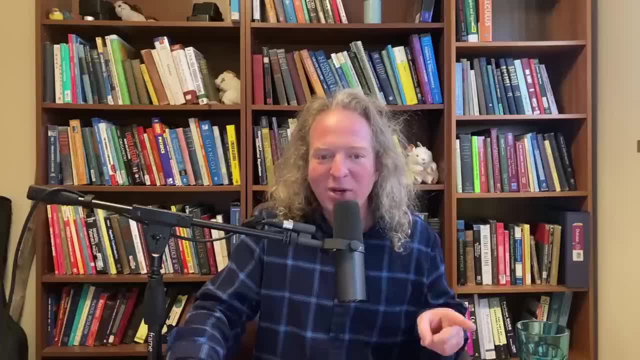 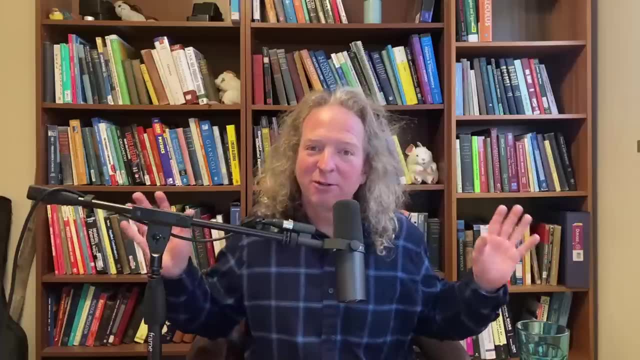 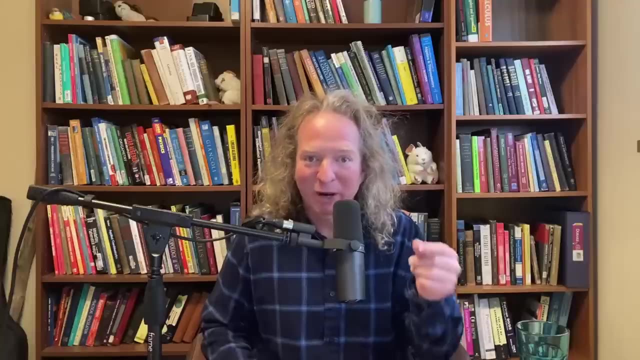 it. uh, i feel that all what i am reading is people showing what they know, showing that they know the material. that is not that they are teaching. i agree. i agree, even even a great book, and not to knock the book, it's a legendary classic, even a book such as, uh, principles of mathematical analysis by rudin, baby rudin. 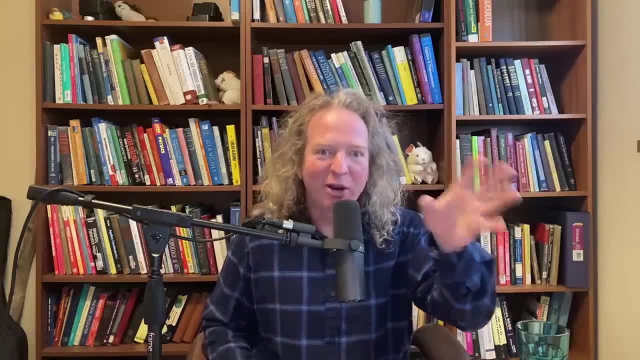 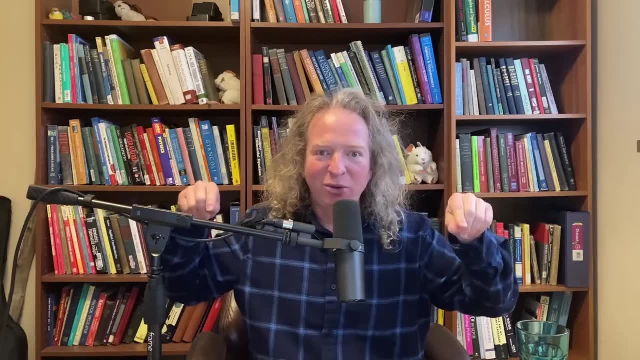 you know, in the proofs it'll say: you know, let epsilon be greater than zero, put delta equal to the minimum of, and it's got like some random insaneness. and they never tell you how to get that. it's like, yep, i know how to do it. this is the delta and it's. 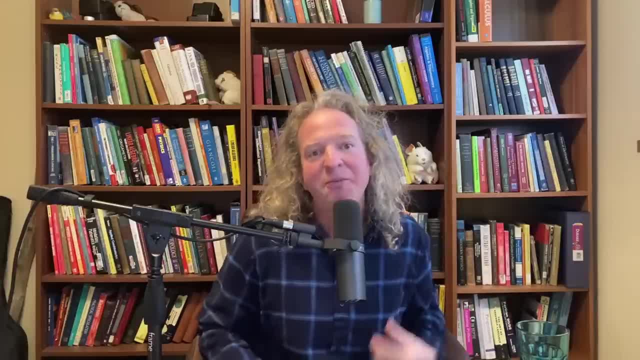 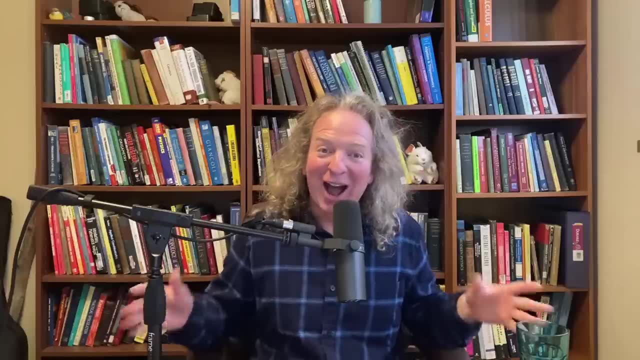 and it works. but i'm not going to show you how to do it because you got to figure it out and i think that's the attitude that a lot of the books take. whether it's the right or the wrong attitude, i'm not going to judge. i personally think it makes it harder. i think it's better to 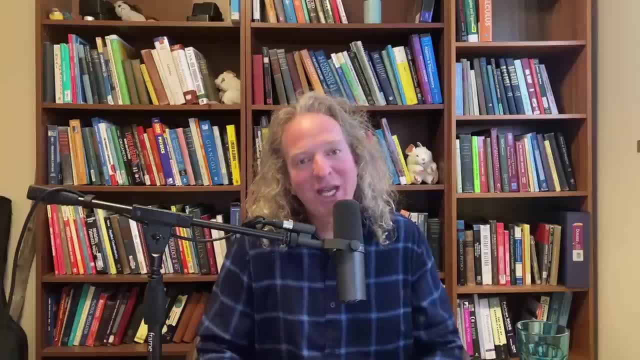 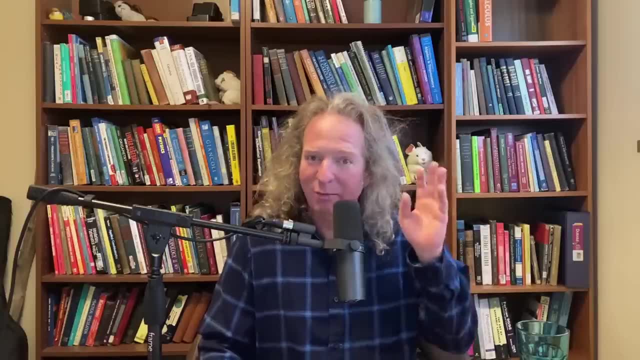 explain stuff, um, but just do the best you can, get as many books as you can and do as many problems from different books as you can, and it helps. it helps even i have a personal experience with this when i took my uh final exam in in measure theory. 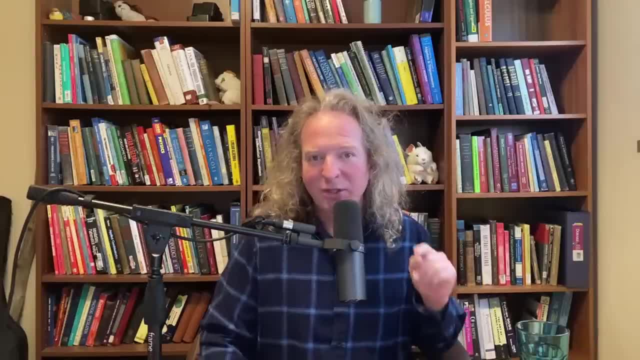 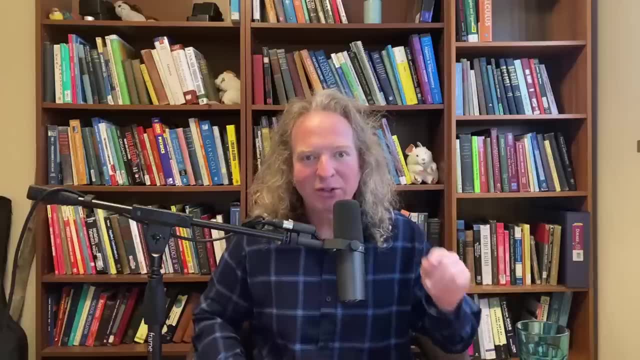 uh, on the final there was a question and i believe i was the only person in the entire class to get it right. i know this because i went to see the teacher for another reason after class and i was the only person in the class, according to the teacher, to get this question in the final exam right and 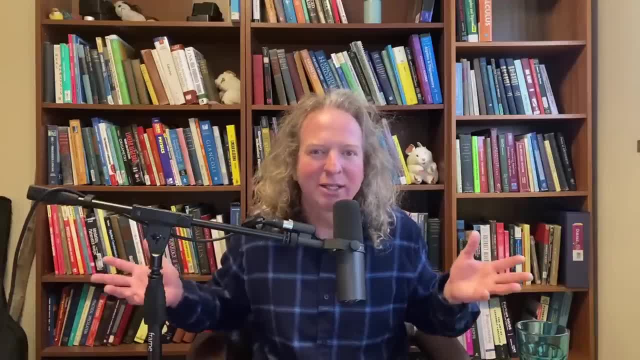 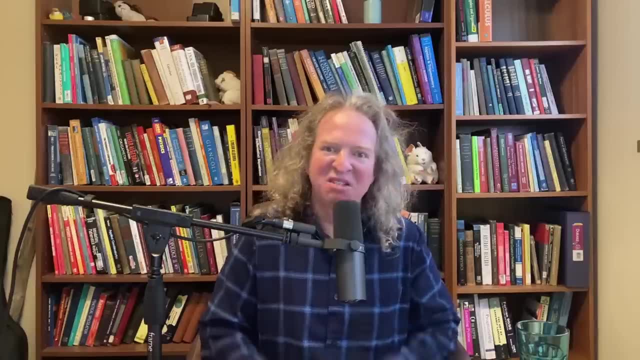 because of that, you know, i got a decent grade. i think i got like an a minus and i think it's because of that that i got an a minus. and the reason i got it right is not because i'm smart. no, has nothing to do with intelligence. what it has to do with is effort, and it has to do with